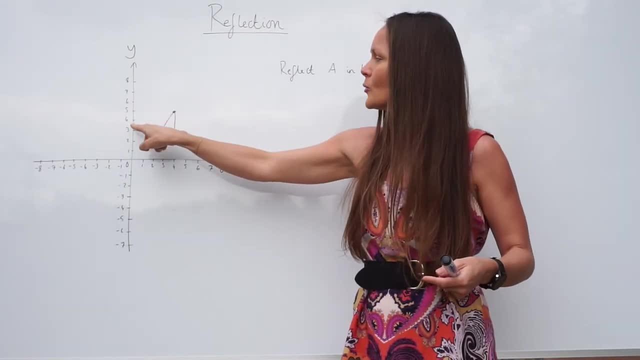 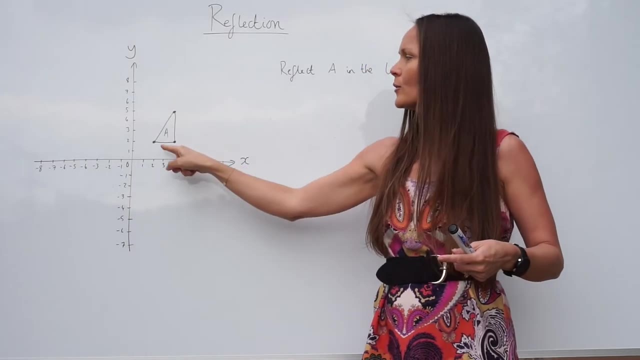 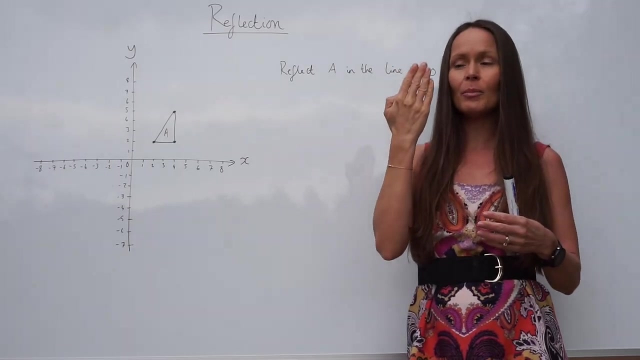 axis. If you look at the Y axis, the X value is always 0 along that line. So there's X equals 0. So we need to reflect this triangle A in that mirror line, the Y axis, or X equals 0. And when we do that, what happens is the shape flips across that line, So it's the. 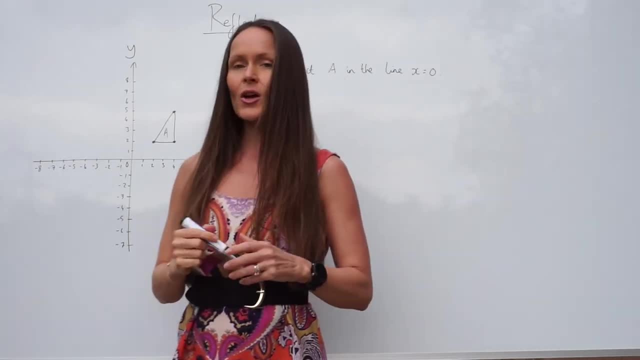 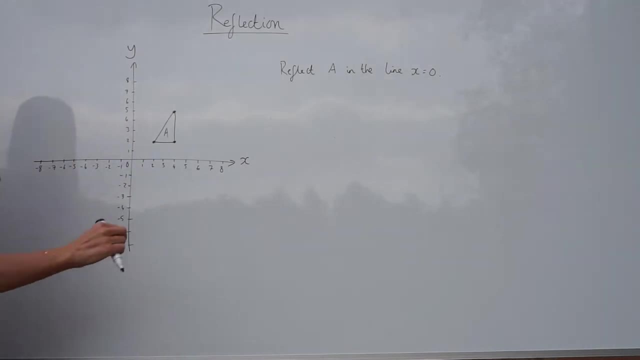 same shape. it's the same size, but it flips across the mirror line. So when you do a reflection, it's a good idea to take one of the points on your shape, It doesn't matter which one. So I'm going to take the bottom left-hand corner here. 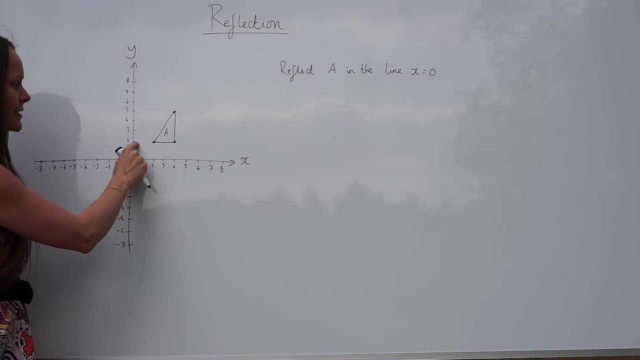 Can you see that it's exactly two units away from the Y axis horizontally. The new point, the reflected point, should be two units, but on the opposite side of the mirror line. Okay, so it should be here. Okay, so they're exactly the same distance away from the mirror line. 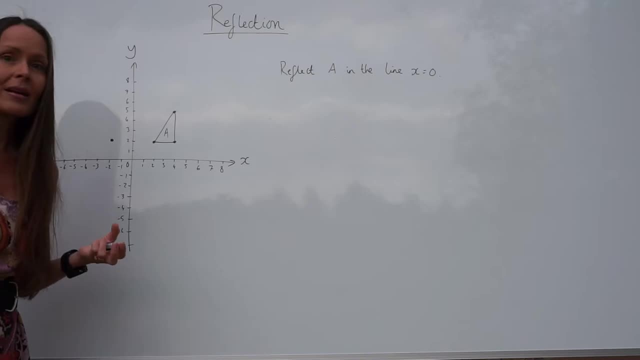 Okay, those two points. Then you can just do the same thing for all the other points. So this point here is four units from the mirror line. So if you count 1,, 2,, 3,, 4, 1,. 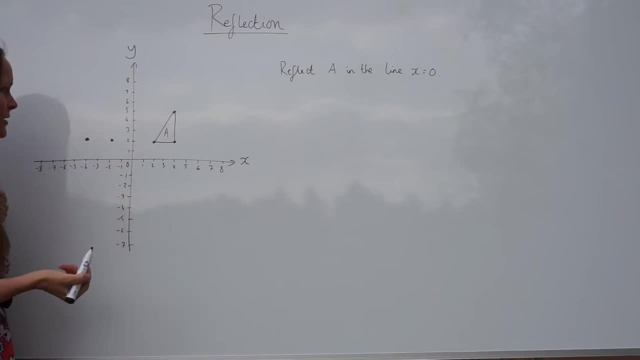 2,, 3,, 4, you have the second point. Then the point up here is also four units away from the mirror line 1, 2,, 3,, 4.. So you count four units again. Okay, And can you see now? 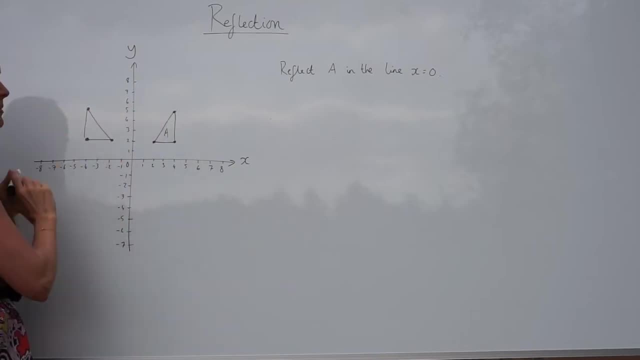 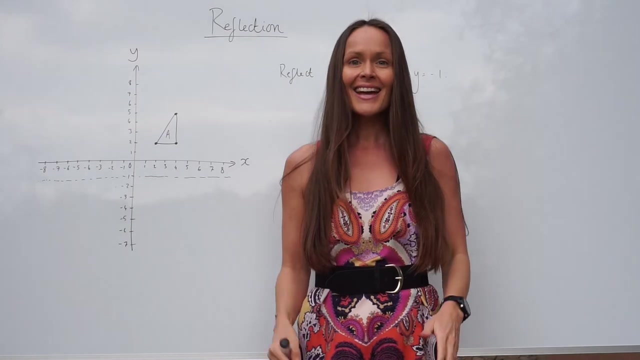 it's the same triangle, it's the same size, but it's flipped in the mirror line. Okay, so that's the image of A. Okay, that's the reflected shape. In the second question it says: reflect A in the line. 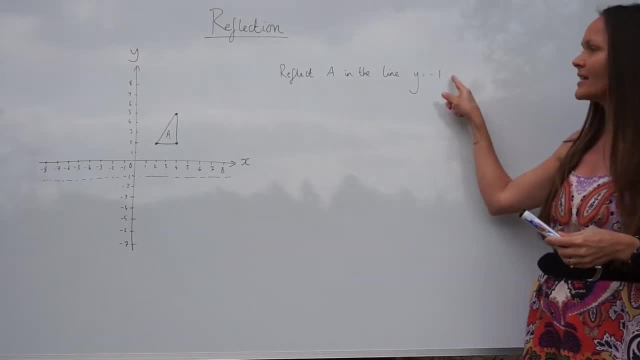 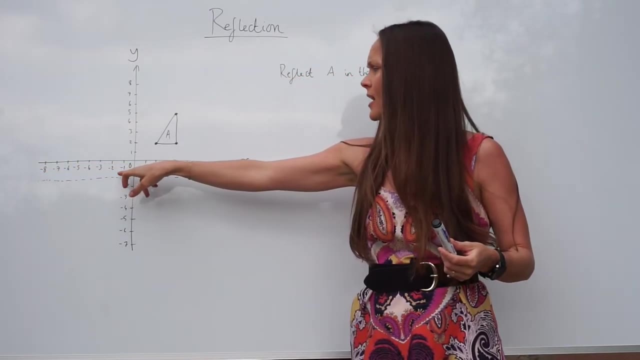 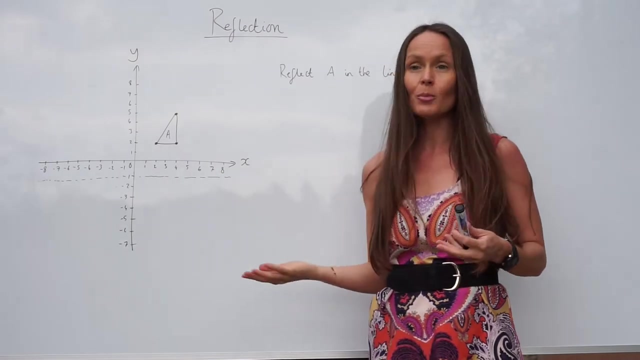 Y equals negative 1.. So if that line isn't already indicated on the graph, make sure you draw it on. Okay, so here I've just marked roughly the line: Y equals negative 1.. Okay, so we need to reflect that triangle in this new mirror line. So the triangle is going. 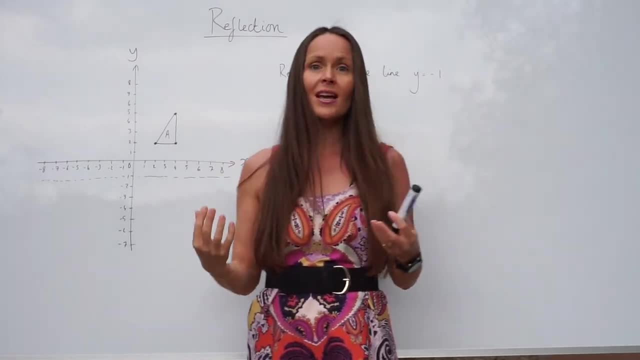 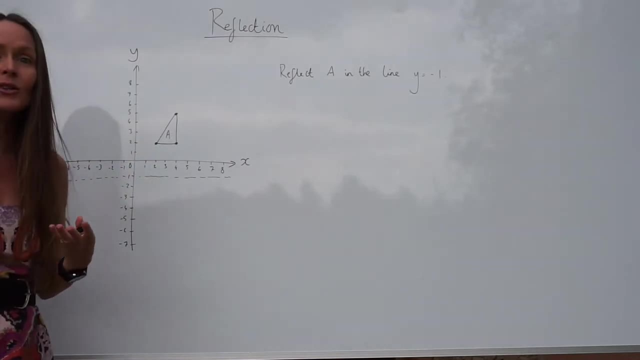 to flip down here somewhere. So, just like before, choose one of the points on your triangle. So I'm going to choose again the bottom left-hand corner and count how many units that point is away from the mirror line. So you should be able to see. this time the point is 1,, 2,, 3 units from the mirror. 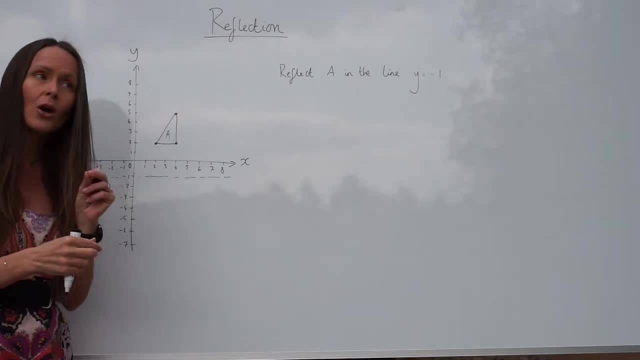 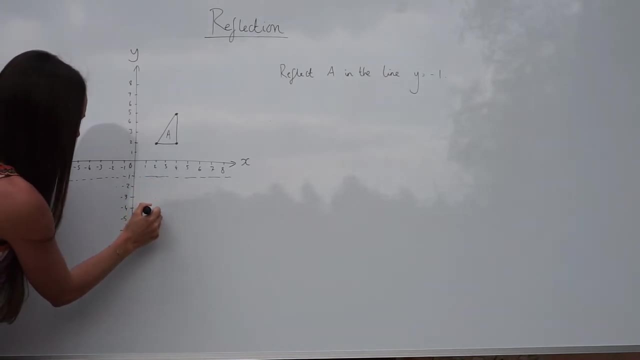 line. So the new reflected point will be three units below the mirror line. okay, in line with the previous point. So I'm going to count 1,, 2,, 3.. Okay, obviously when you do this in an exam question, you'll be a lot more tidy than me when I'm doing it on the whiteboard. 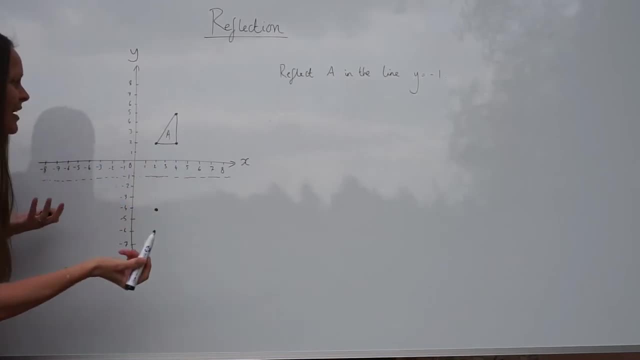 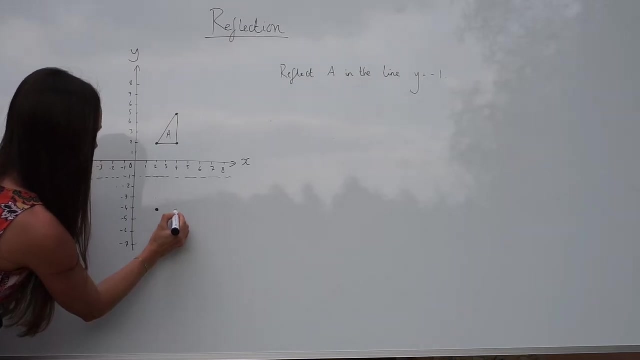 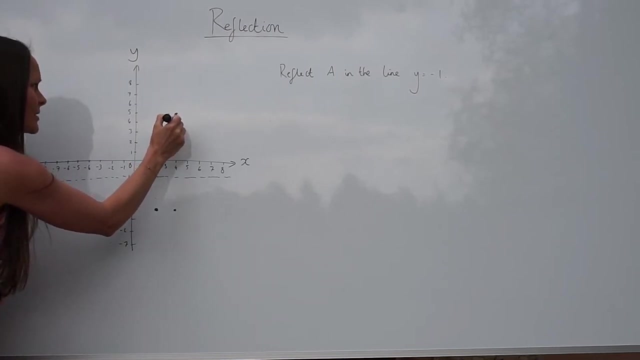 Then for the second point. again, it's three units from the mirror line. So you count three units below 1,, 2, 3.. Okay, so there's the second point. And lastly, the point up here is six units from the mirror line. Okay, so you have to count six units away from the 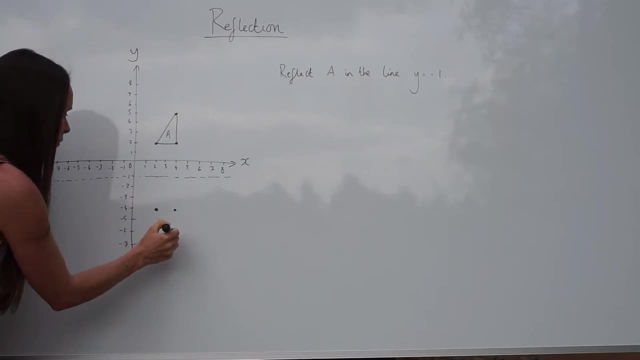 mirror line, So 1,, 2,, 3,, 4,, 5,, 6.. So it takes you all the way down, Okay, so that's the point. All the way down there, Okay. so then you can join up the points And that is the. 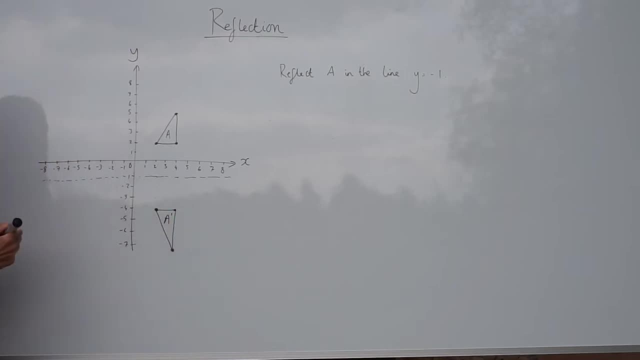 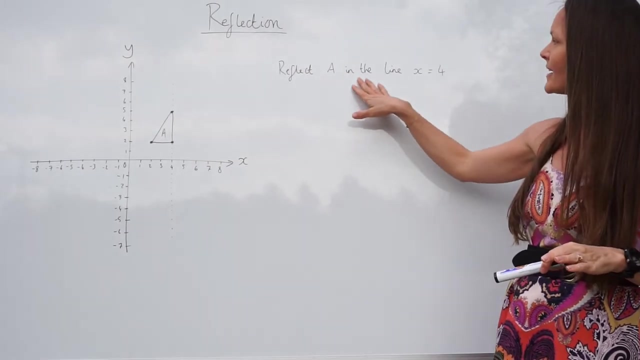 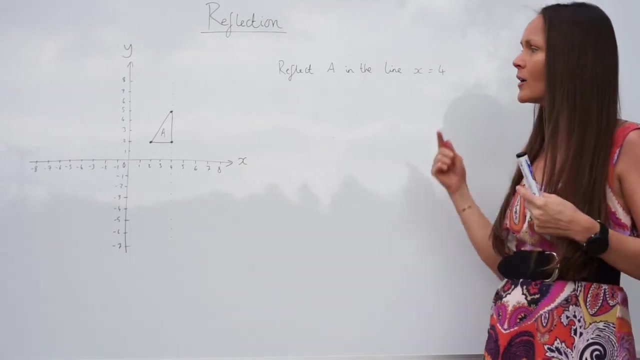 image of A. Okay, we have reflected triangle A in the mirror. line y equals negative 1.. Okay, so next up, we've got reflect A in the line x equals 4.. So, just like before, if the line x equals 4 isn't already indicated on your graph, find it Okay. so I've just done. 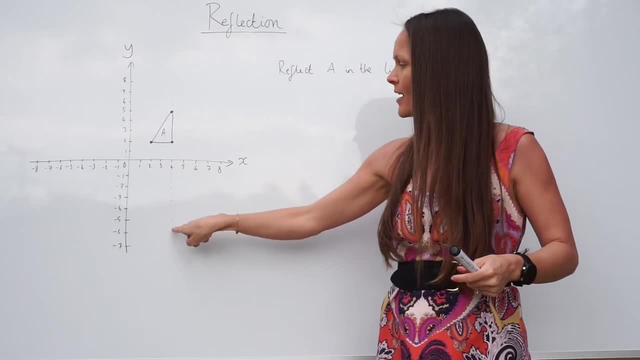 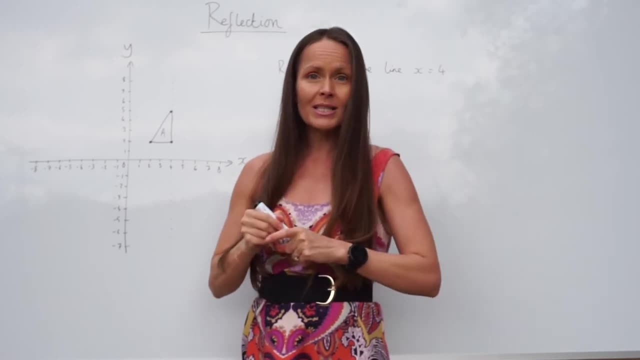 a few dashes here along x equals 4 to show that it's not indicated on your graph. So that line. And so we need to reflect triangle A in that new mirror line. Okay, so it's a little bit different this time, because two of the points are on the mirror line, So when 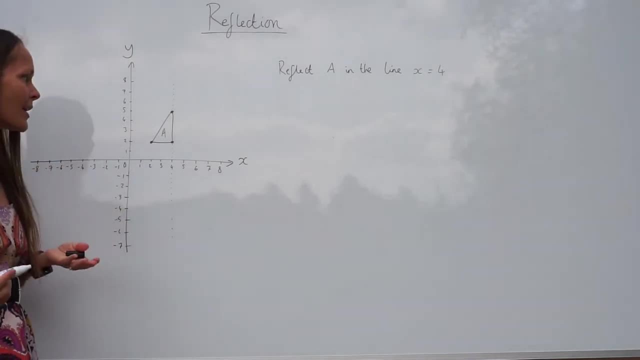 the points lie on the mirror line. they don't move. Okay, they stay where they are. So the only one that's going to reflect, or move, if you like, is this point here. This point is two units away from our mirror line. x equals 4.. So you need to count two units away from. 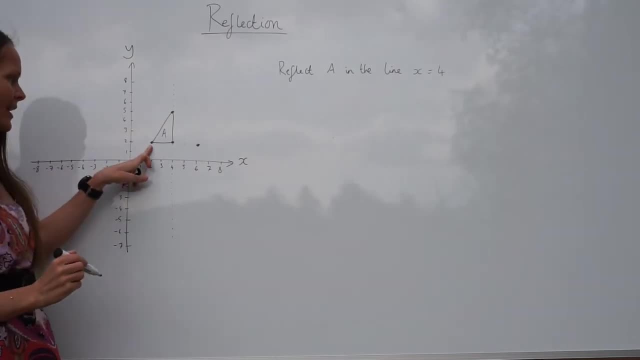 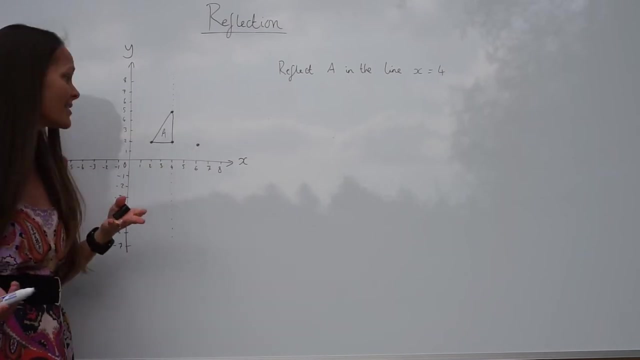 it the other way. Okay, so this point here on our triangle is reflected over here. Okay, it's exactly the same distance from the mirror line, but on the opposite side. So now you can join up the points. Okay, so that is the image of A, So it doesn't matter that it lies. 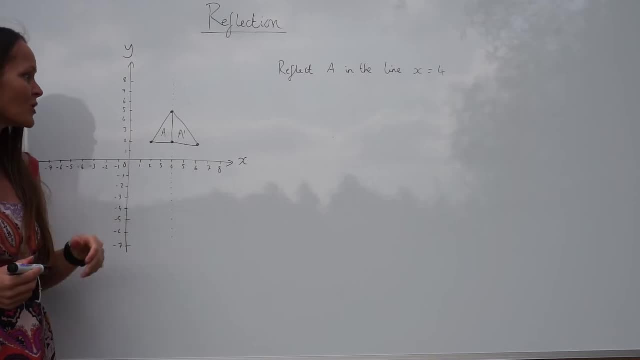 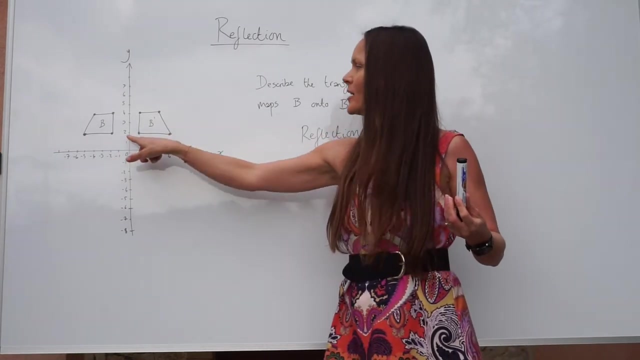 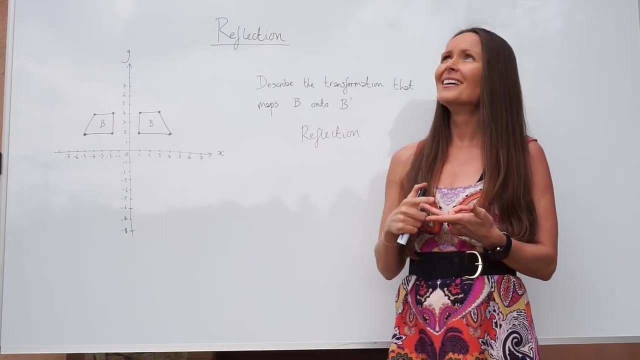 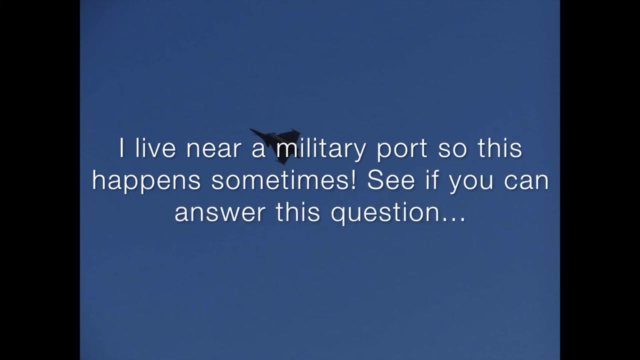 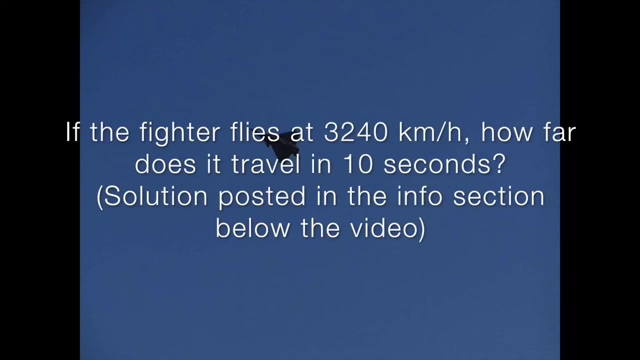 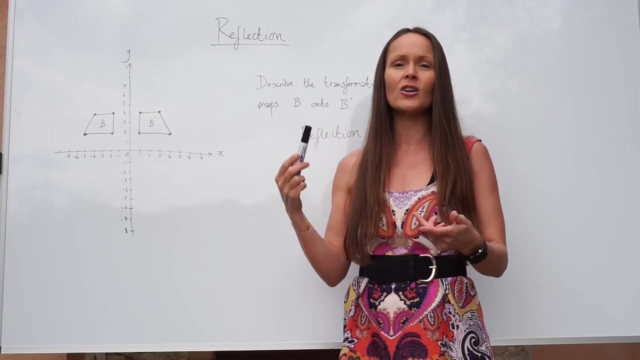 on the mirror line. Okay, we've done the reflection. That is the image of A. In this next question it says: describe the transformation: the maps B Onto B dash. So transformation just means either rotation- Okay, so I'll start again. So transformation just means either rotation, reflection, enlargement. 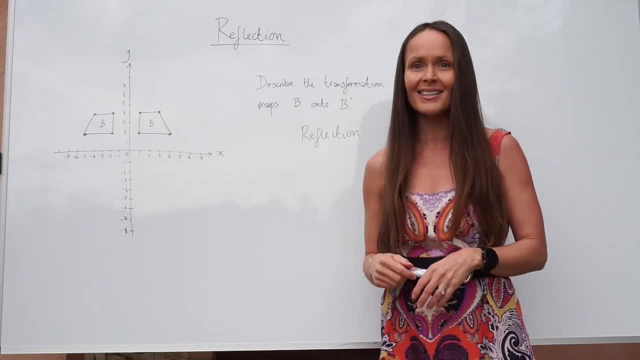 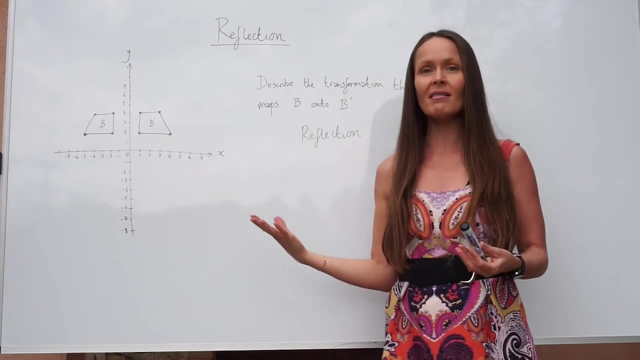 or translation. Hopefully now you should be able to recognize that this is a reflection, because it's the same shape, it's the same size, but B has been flipped in a mirror line. okay, to find the image B dash. So the first thing you would write down for your answer: 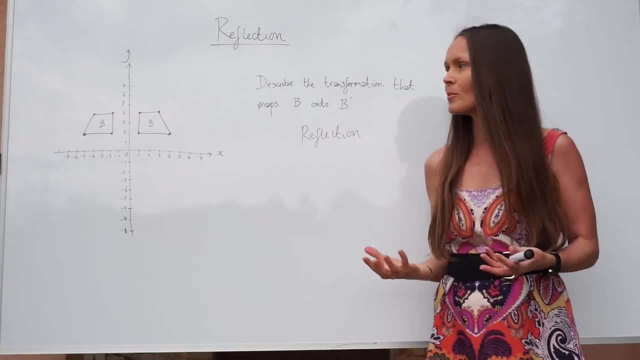 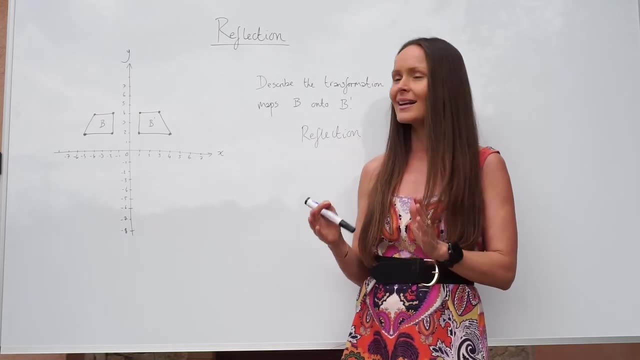 is just the word reflection. Okay, that is the transformation. But to get full marks you need to find the equation. So you need to find the equation, So you need to find the equation of the mirror line. Now, remember, the mirror line is exactly halfway between: 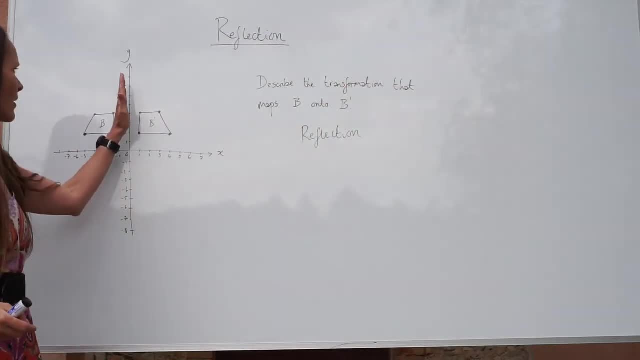 the two shapes. Okay, so it's going to be here somewhere. Okay, but we need to find it precisely So I can see between these two points there are exactly three units between them. If we half three, we get 1.5.. So you need to count 1.5 units from here to find. 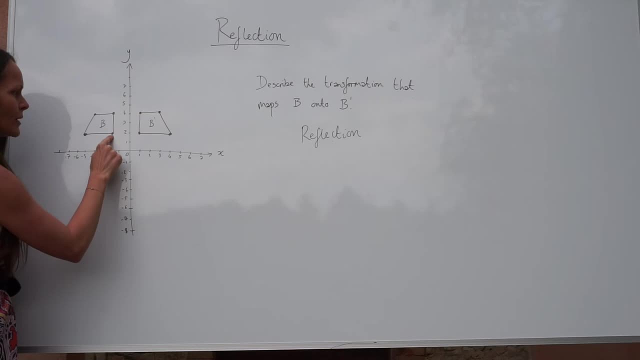 the mirror line. So this is at minus 2.0. And this is at minus 2.0. And this is at minus 2.0. So if I add 1.5, it takes me to negative 0.5.. Okay, so it's in between a square, but 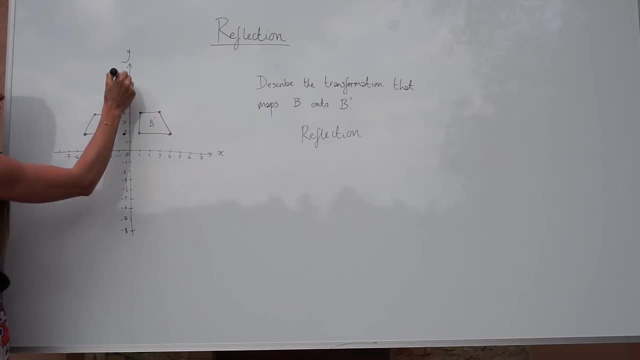 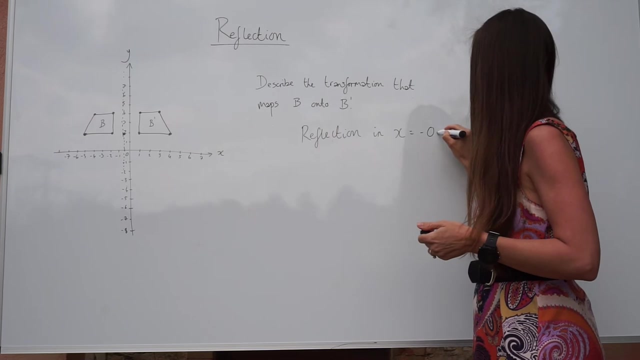 that's fine. So there's negative 0.5.. So the mirror line is there. Okay, the mirror line or the equation of the mirror line would be: x equals negative 0.5.. Okay, so you can write the final answer like that. It's a reflection. 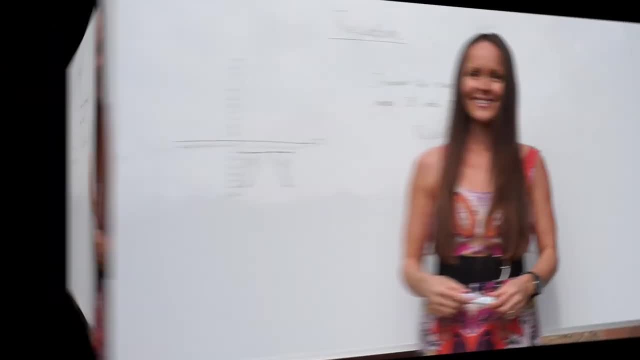 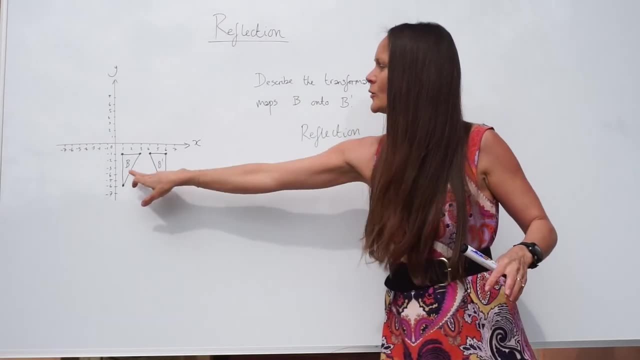 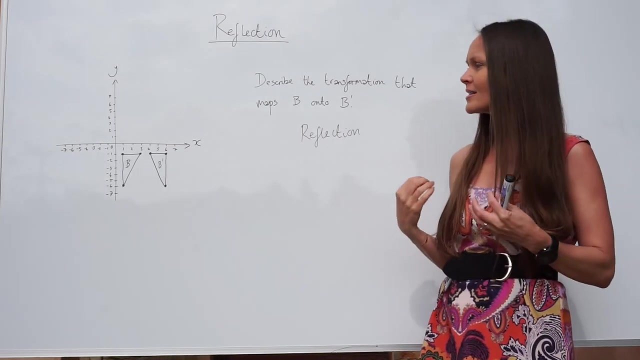 In x equals negative 0.5.. So, just like in the previous question, we have to describe the transformation that maps B onto B dash. So the first thing you would write down in this question would be reflection. Okay, we know it's a reflection, it's the same size.